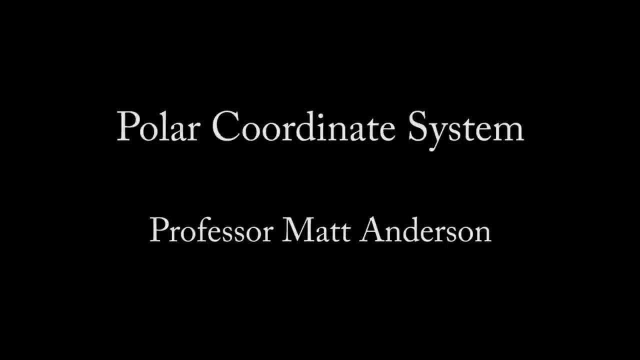 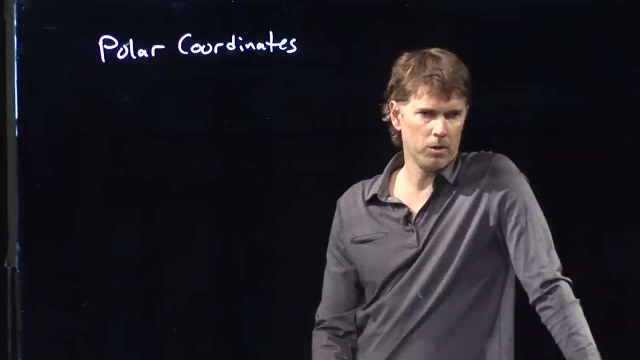 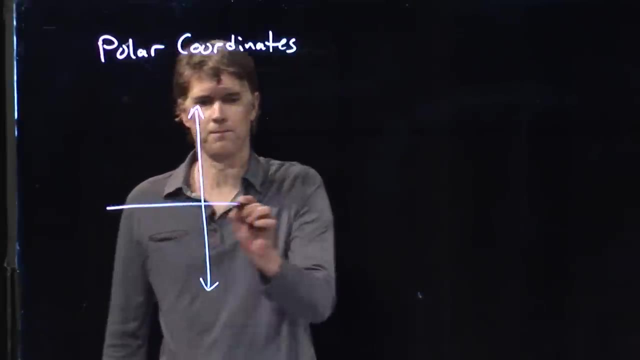 Hello class Professor Anderson. here One of the coordinate systems that you need to be very familiar with is polar coordinates, So typically we're only going to worry about two dimensions. A lot of the motion that we deal with is just two dimensional, So we can. 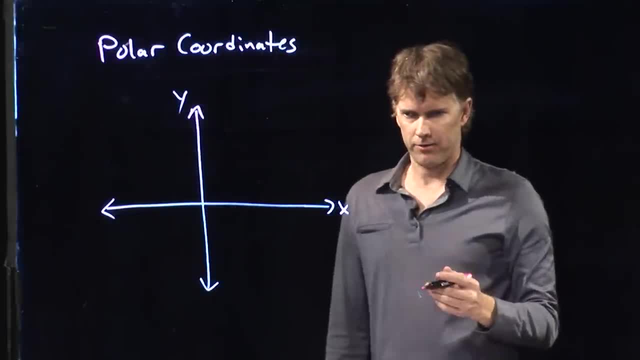 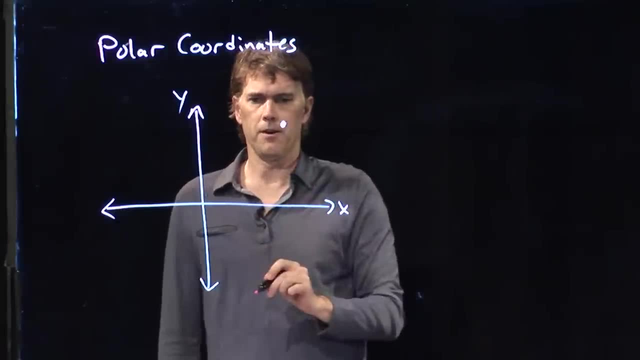 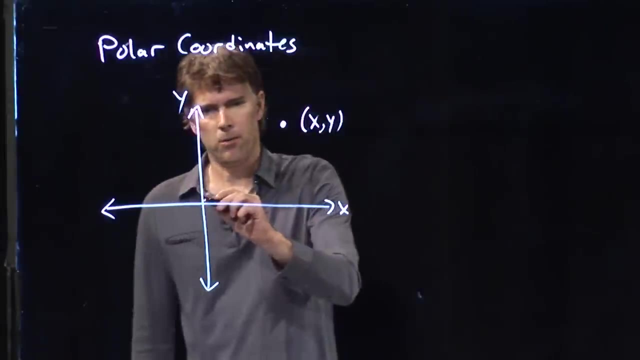 have an x- y coordinate system. That is of course our good old Cartesian coordinate system just collapsed into two dimensions. But let's say I have a point out here And I know that it has some x- y coordinate in that Cartesian space. But now I want to define that in terms 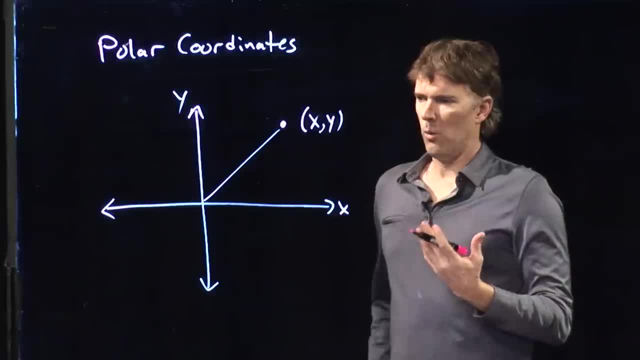 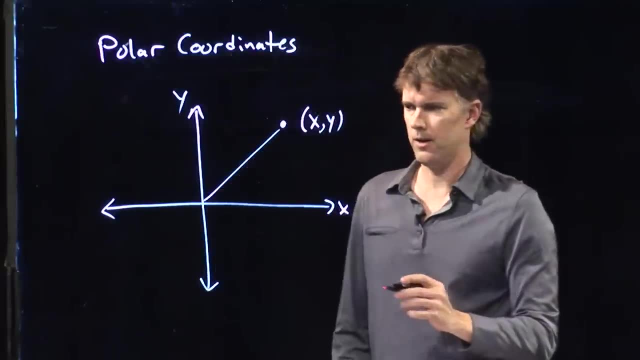 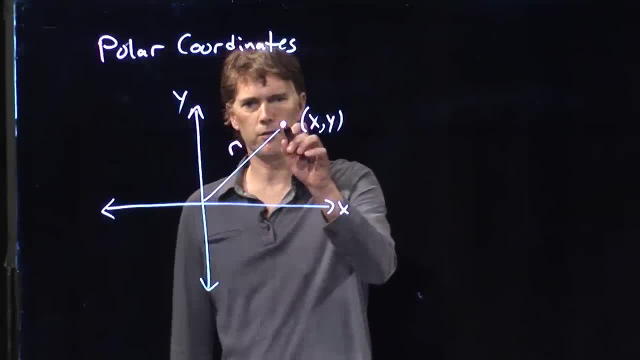 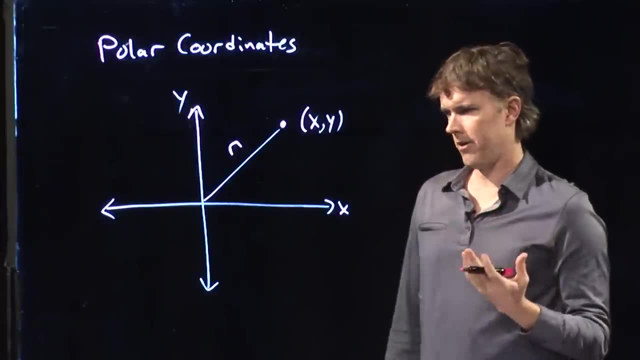 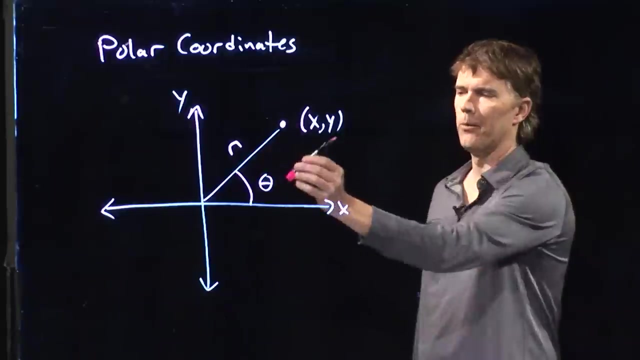 maybe is enough, but not quite right, Because if I just told you r, you could be anywhere on a circle of that radius r. So we need one more variable, And the variable that we're going to use is theta. What's the orientation of that line with respect to the x axis? And 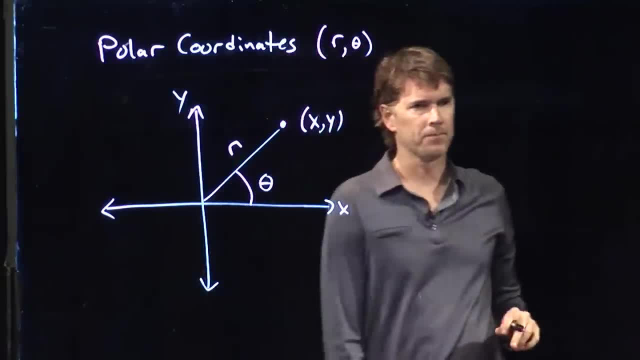 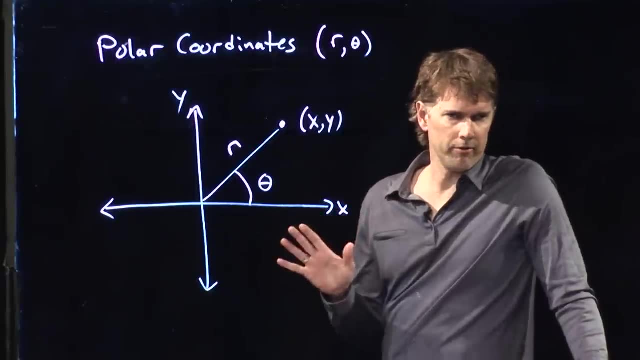 so these are called polar coordinates, r and theta To be technically correct. the three coordinate systems that you need to be familiar with are x, y and theta, So what we're going to need to worry about as you go further in physics are the Cartesian coordinate systems. 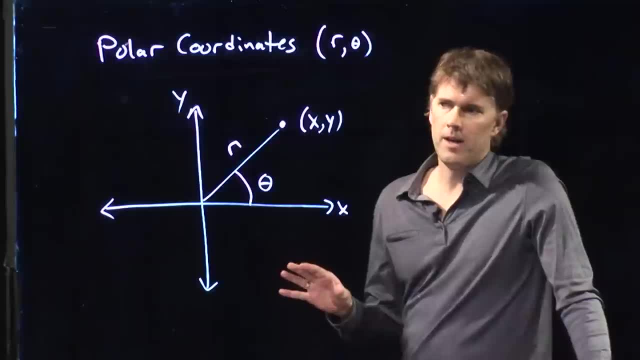 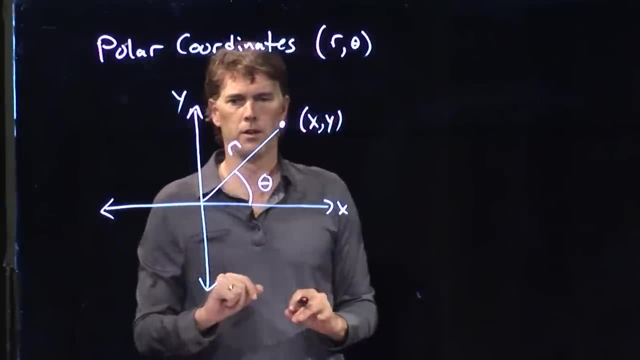 cylindrical coordinate system and spherical coordinate system, And this would correlate more towards the spherical coordinate system, But in two dimensions. we call it polar coordinates. How far are you from the origin? That's r. What's your angle relative to the x axis? That 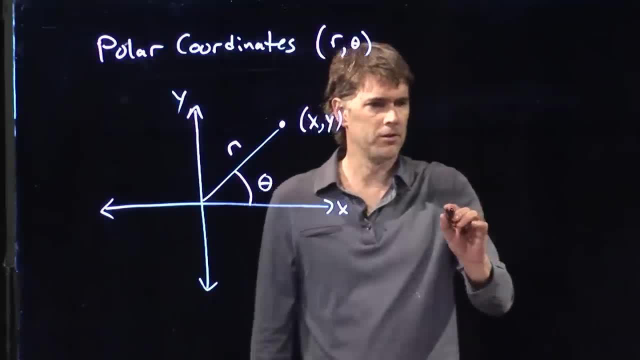 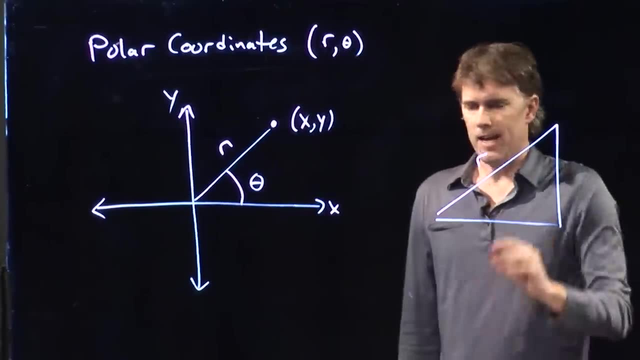 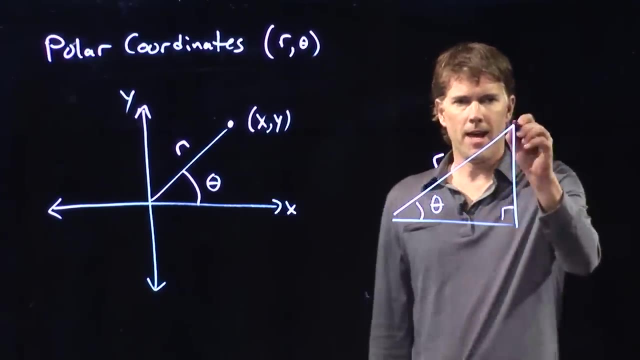 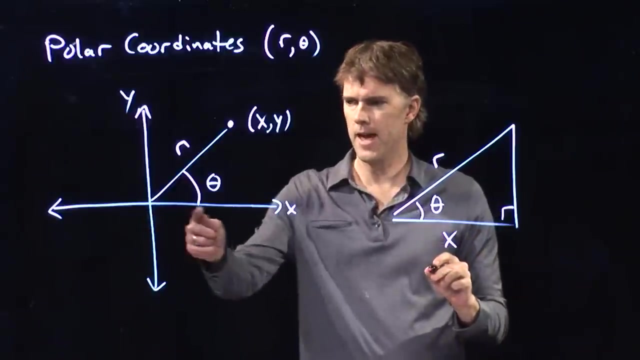 is theta. And now you can see what happens. There is a nice little relationship between these things. So if I draw that line again, I complete the triangle, make this a right angle and this is theta. then that x- y coordinate up there corresponds to what Corresponds to moving over in x by that amount Moving up in y.